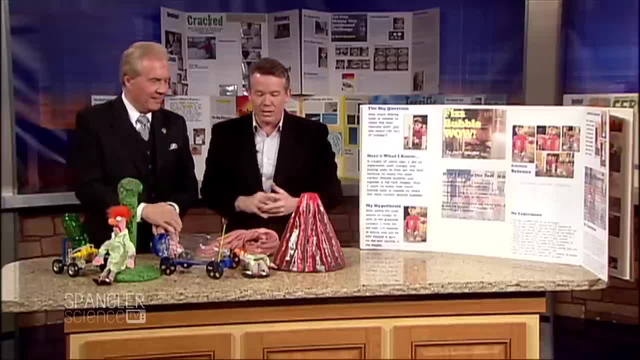 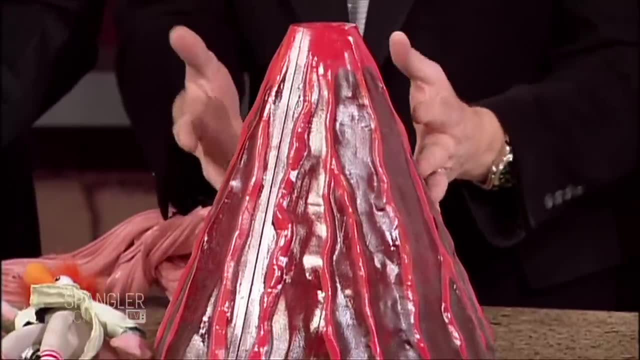 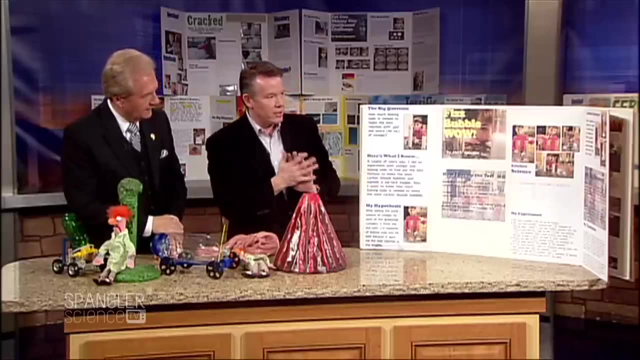 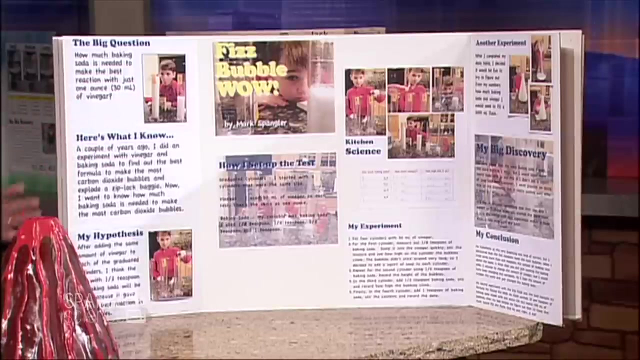 So, for example, I brought the Alka-Seltzer, One of our favorites. This is just a teacher's nightmare, because you look at it and go, oh, we're not going to get a science project, We're just going to get a demonstration. And you're right, If you just mix vinegar and baking soda, everybody knows what's going to happen. So let me point you to the board right here. So I'm showing you some things our little guys have done over the years. So look at this: A fizz bubble. Wow, This is a test. now to say if I want to make the vinegar baking soda, why don't I have some variables? Why don't I try two tablespoons of vinegar? 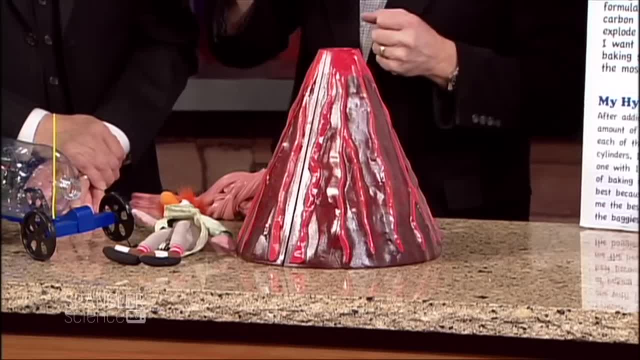 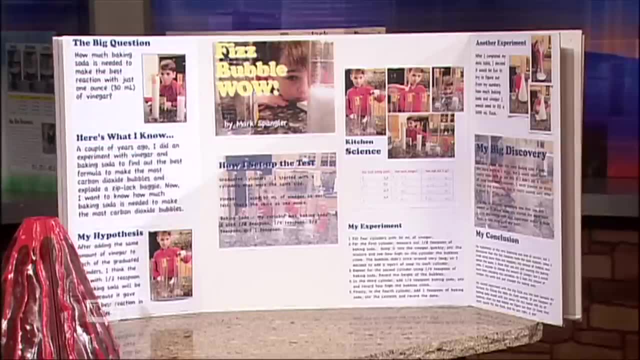 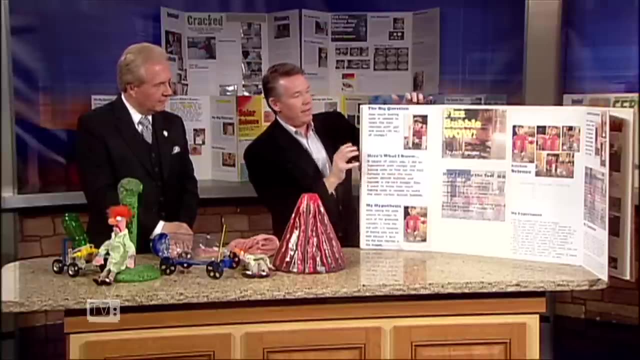 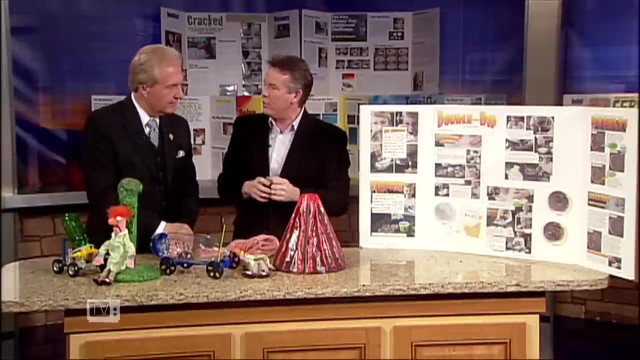 Two tablespoons of baking soda and three tablespoons of baking soda, Four tablespoons, Same amount of vinegar. See which one gives us the biggest rise. Now it's a science project. Bingo, because now I'm counting, comparing, classifying, observing, measuring- Easy to do. Now, when I get to this, I at least have some data. that kind of goes. there. I feel like the old Leno show. You know how everybody loves to grow bacteria. So we've done that before. where I walk around the newsroom and find the dirtiest thing, Yes, and unfortunately we found a lot. Yeah, that's exactly right. So in 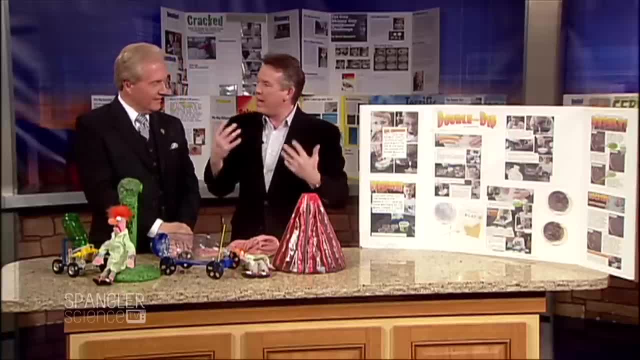 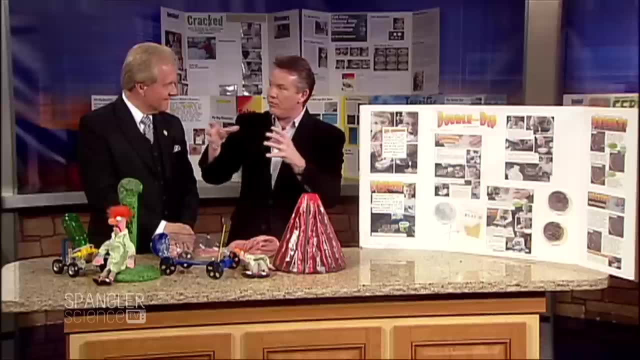 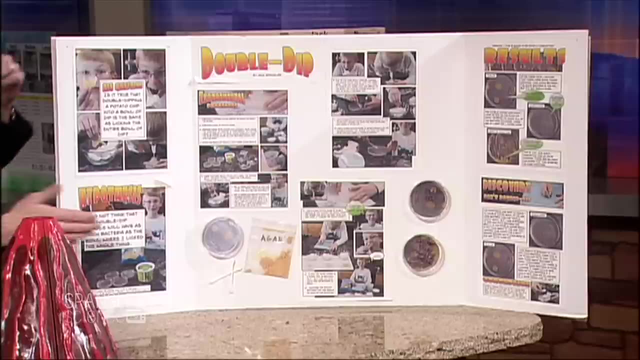 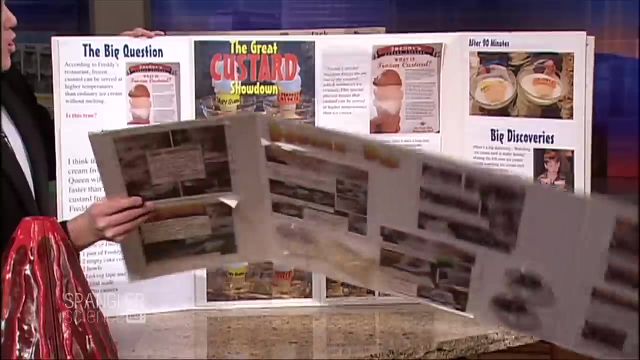 those keyboards are dirty and so forth. but that's not a science fair project. Just finding it doesn't actually do it. So that that doesn't do it, Why don't we now take that and now use that data to go find something else? For example, little Jack Spangler decided years ago, if I double dip a chip, is that really going to spread bacteria? And so he used this as a way to be able to see whether or not the bacteria grows. Yuck, That's exactly what you don't want to do. No double dip. Little Mark decided that he was going to do this. They said that at Freddy's. 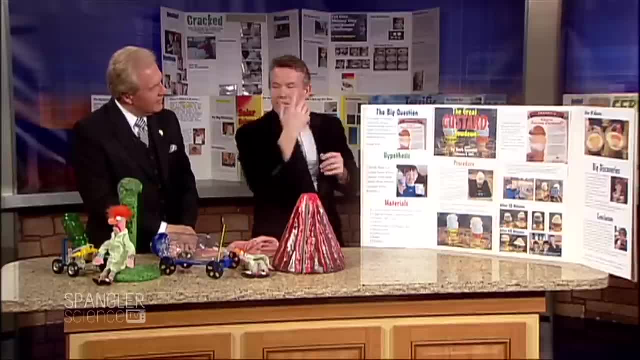 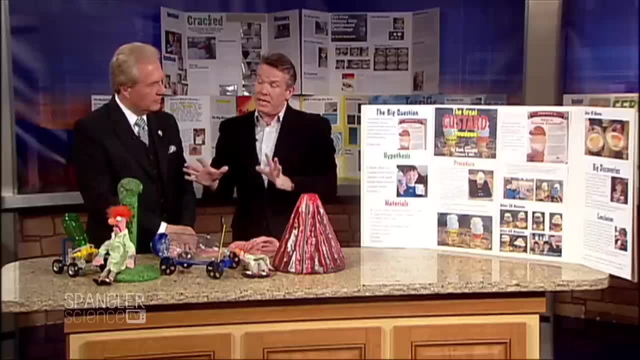 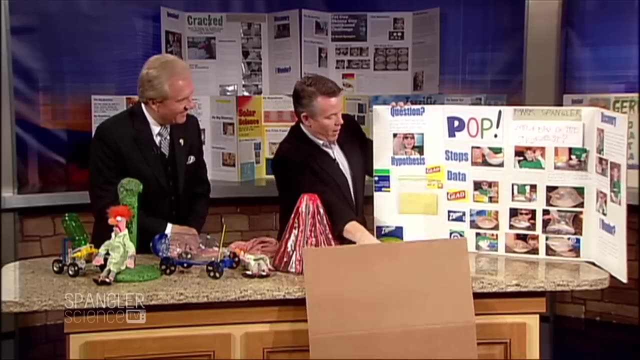 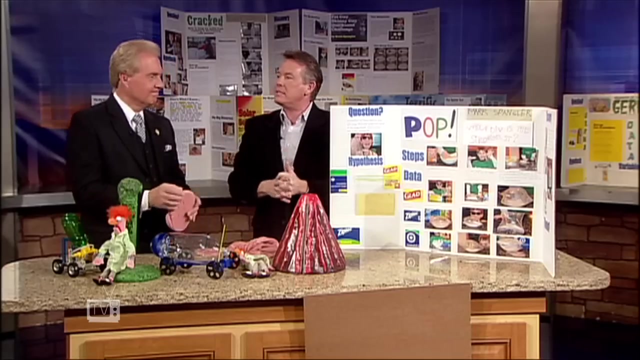 College. The custard doesn't melt as fast as Dairy Queen, And so you set up the comparison. Great, That's a science fair project versus just doing a little demonstration and activity. So this science fair one on one dot com: You're going to be able to download all the things that you need to do so that in the kitchen you can sit there and just see why things will explode and test different Ziploc bags and vinegar, baking soda, whatever it is. But make it fun and you'll change the way kids think about science. for a question, The discovery, The answer: Phenomenal. I'm going to put this science fair one on one. One dot com You got it. Thank you, Science guy.